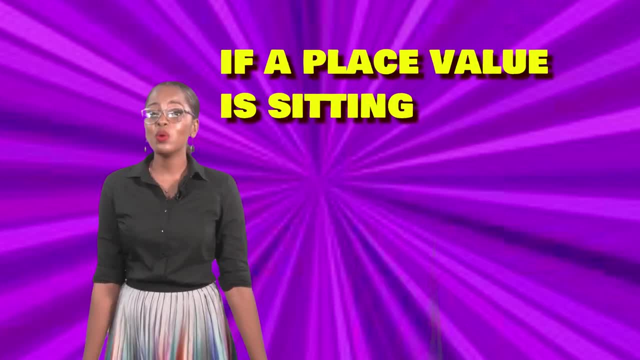 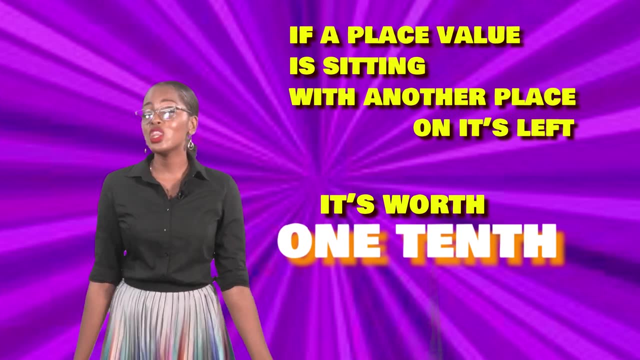 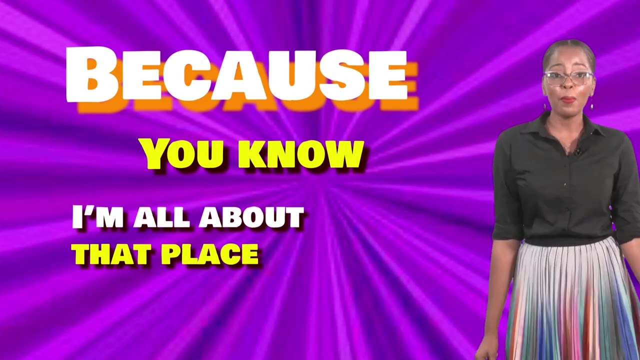 Mm-hmm, And if a place value is sitting with another place on its left- Mm-hmm- Then it's worth exactly one-tenth, no more, no more, no less. Oh, because you know, I'm all about that place, about that place, place value, I'm all about that. 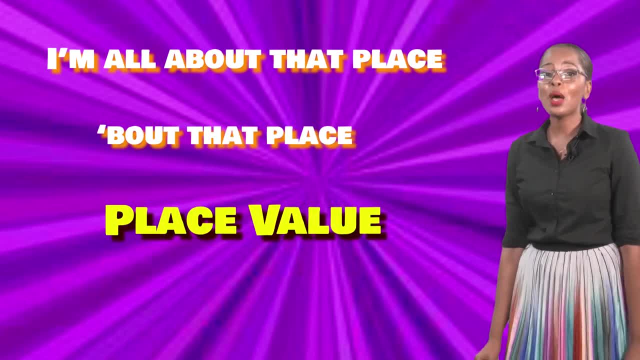 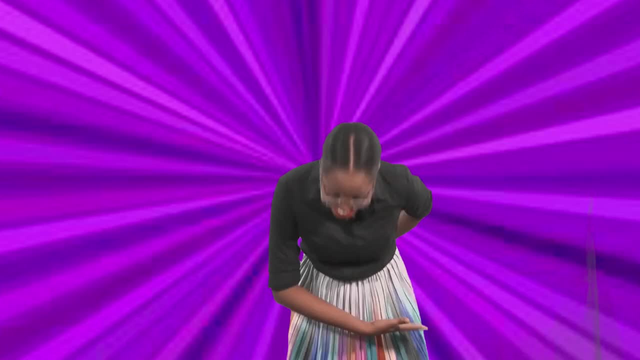 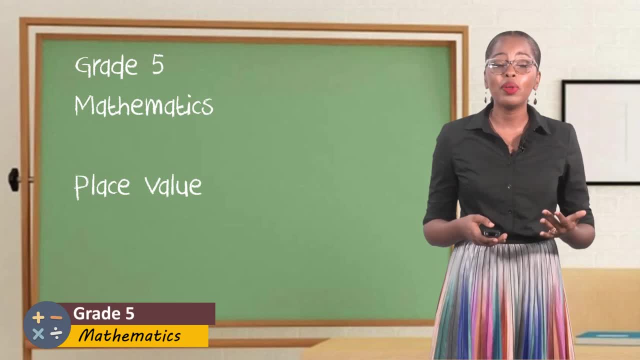 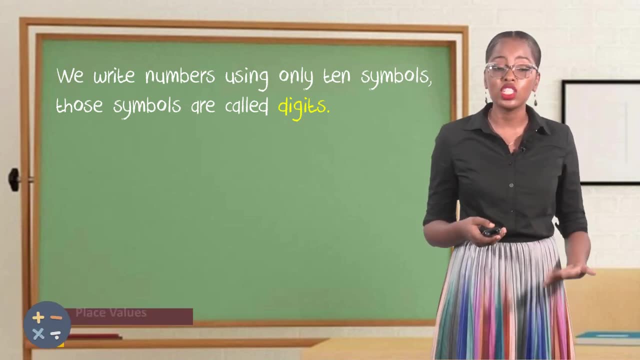 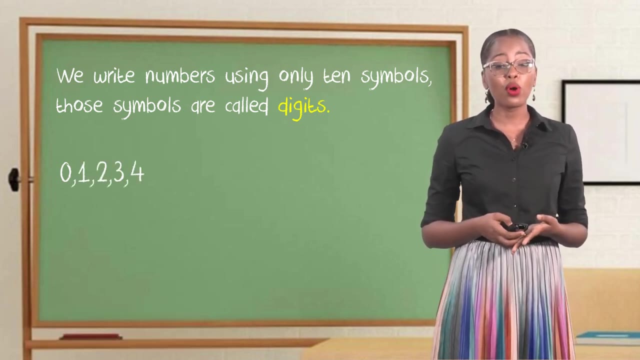 Okay, boys and girls, Now let's move on to discussing what place value is. We write numbers using only ten symbols. Those symbols are called digits. The digits we use today are zero, one, two, three, four, five, six, seven, eight and nine. 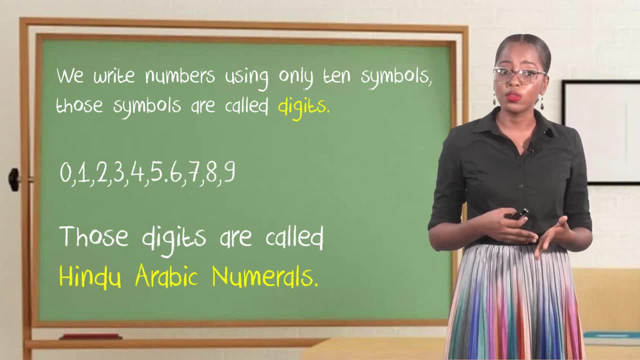 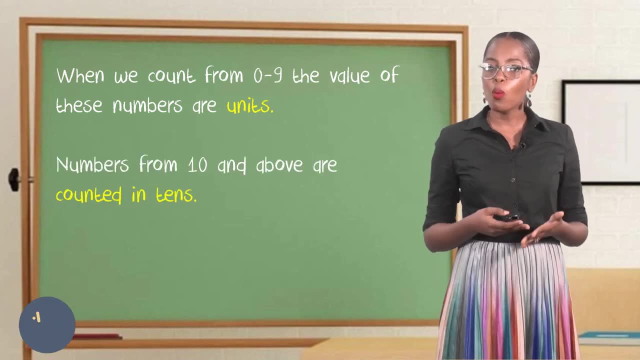 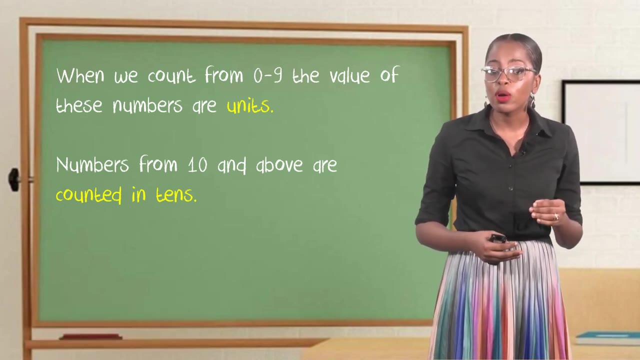 Those digits are called Hindu Arabic numerals. When we count from 0 to 9,, the value of these numbers are units. However, when we move on to count numbers that are 10 and above, the value of those numbers changes as well. 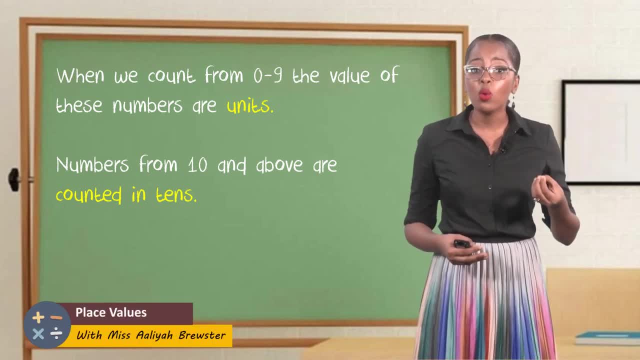 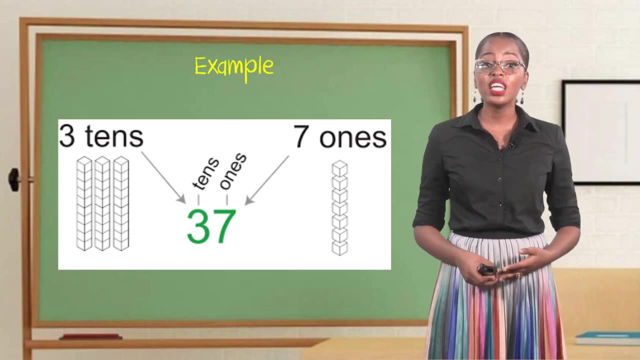 We are no longer counting in units but now we are counting in tens. For example, suppose we have the number 37. 37 has two digits, 3 and 7.. In 37, the 3 is taking up the place of the tens. 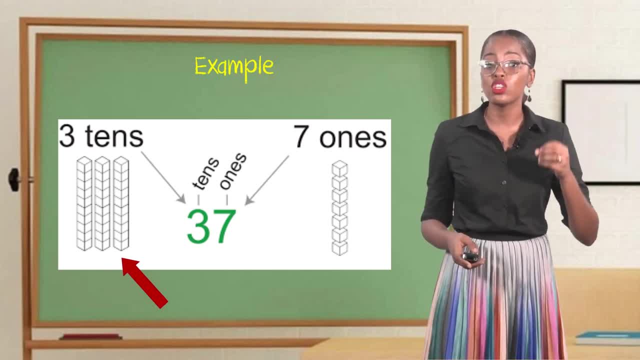 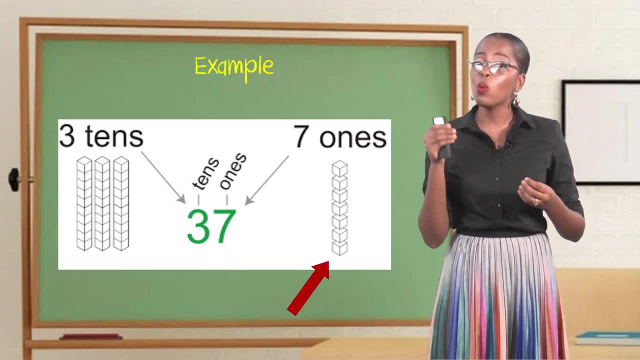 which simply means that 3 tens make 30.. On the other hand, the 7 is taking the place of the 1s, which means there are 7 1s being added to the 30. So when we add 30 plus 7, we would get 37.. 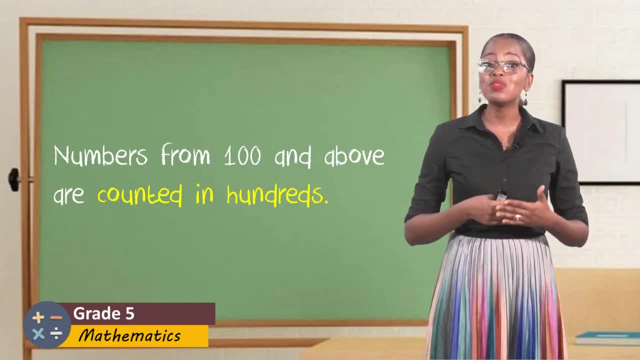 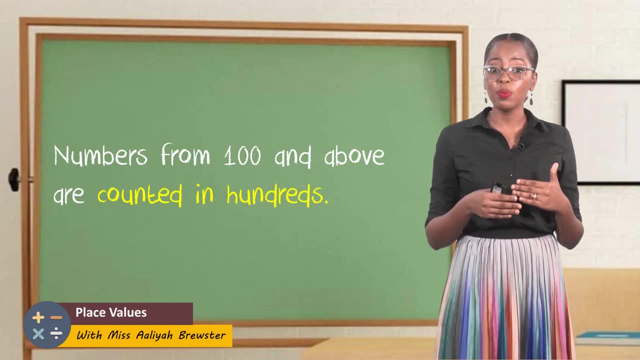 Now, boys and girls, let's look at the numbers. Once we would have counted up to 99.. So, from 10 to 99,, 100 comes after 99,, obviously, And now we can say we are in the hundreds place value, For example. let's look at the number. 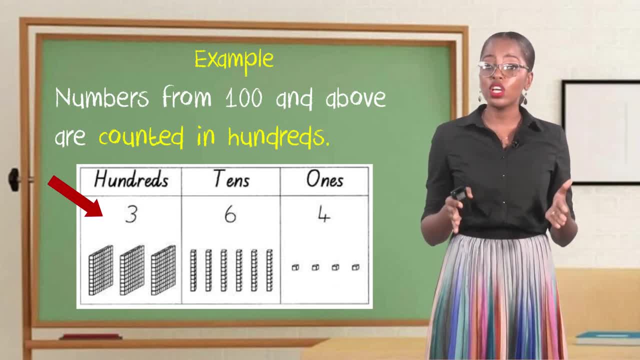 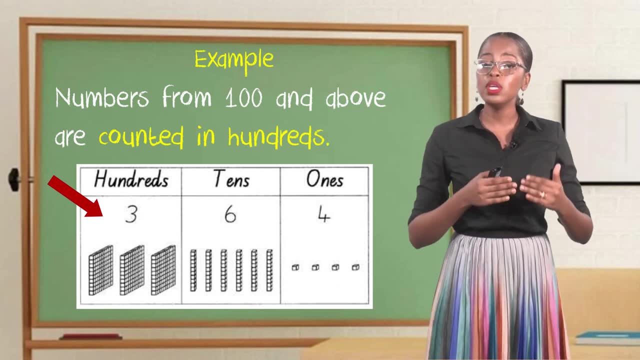 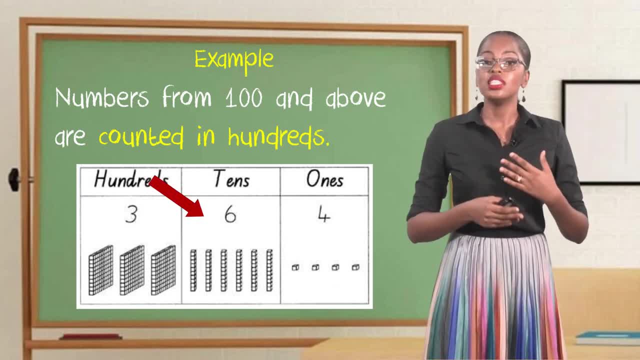 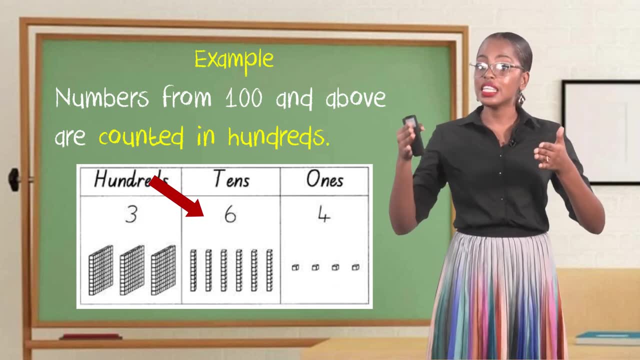 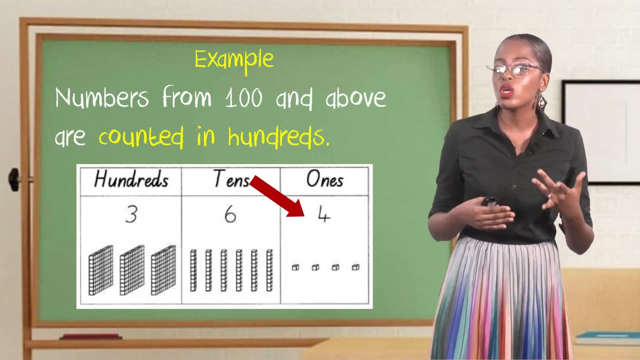 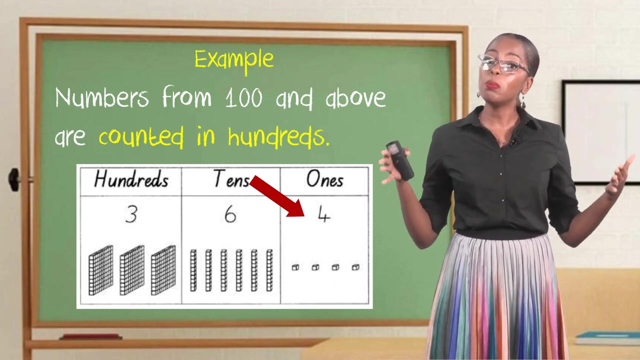 three hundreds in it, while tenth takes up the place of the tens column, which simply means that 60 makes up 364 or six tens. and finally, the four takes up the place of the four columns, which means that four units or four ones is being added to 360 to make up the number 364. 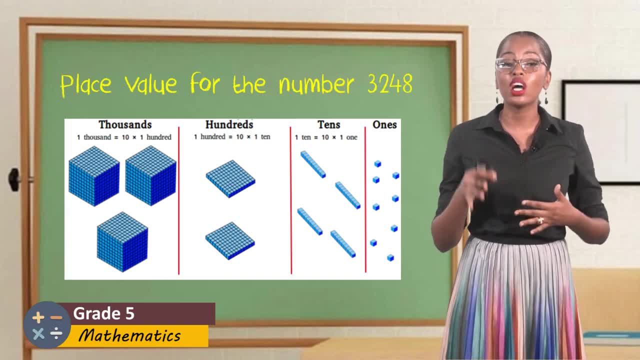 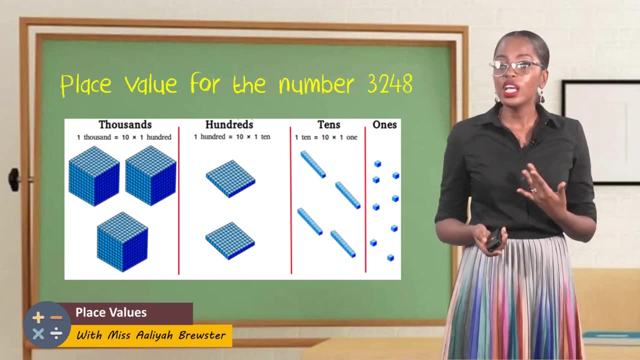 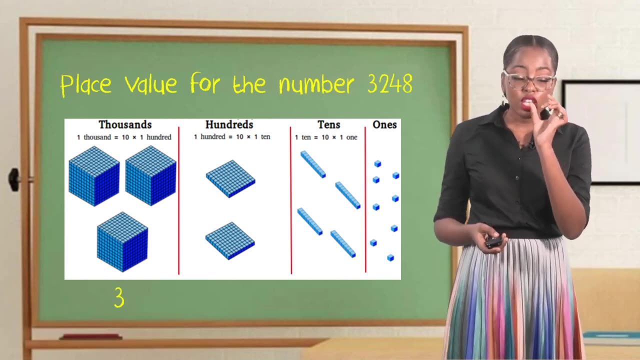 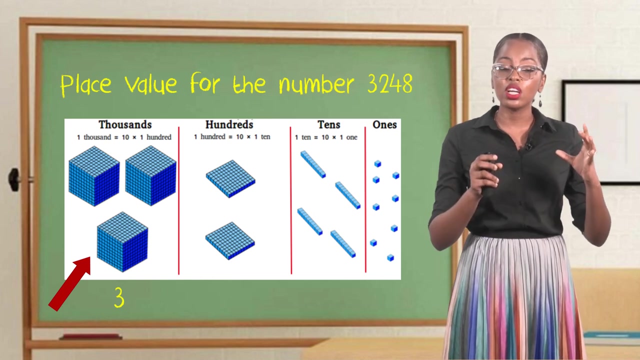 okay, boys and girls, let's move on to discuss the thousand place value. the thousand place value starts from the number one, thousand. for example, let's look at the number three thousand two hundred and forty eight. in that number, the number three represents the thousand place value and if you look at the picture, thousand there is symbolized by three large cubes. 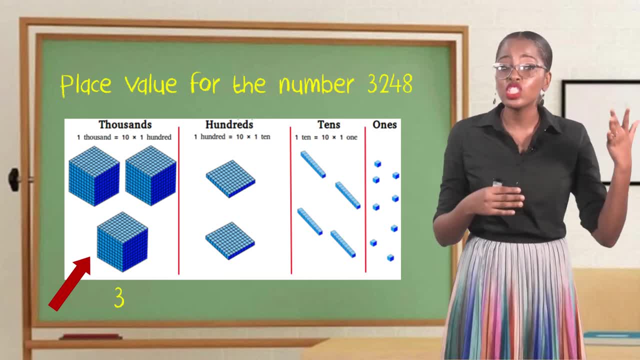 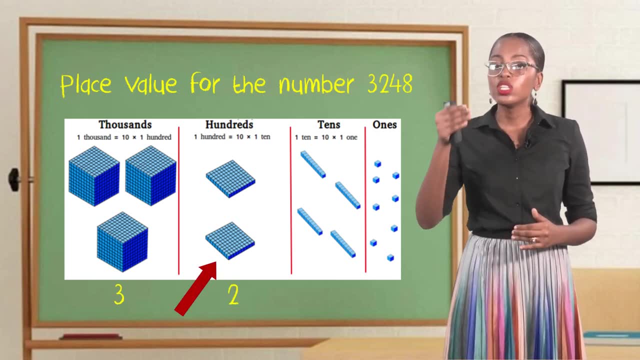 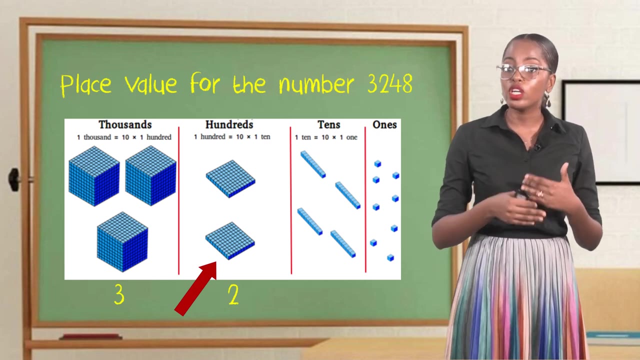 that simply means that the value of three is not just three, but in fact it is three thousand. Now we look at the two. The two is represented by hundred, and that simply means that two hundred makes up the number three thousand, two hundred and forty-eight. So, boys and girls, we know that four is in the 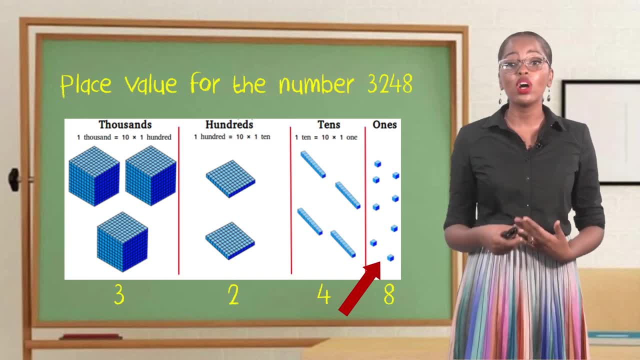 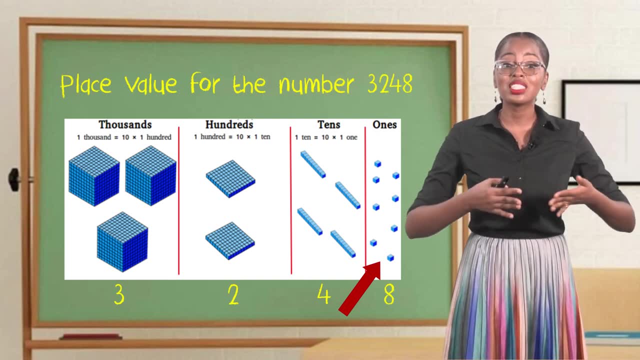 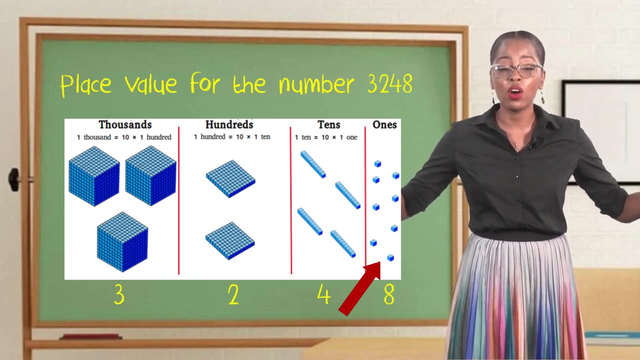 tenths place value column, while eight is in the ones place value column. but numbers don't just stop at thousands. You should know that numbers can get as huge as this entire planet or this world. They go on and on right. So after one thousand, the next place value, moving to the left. 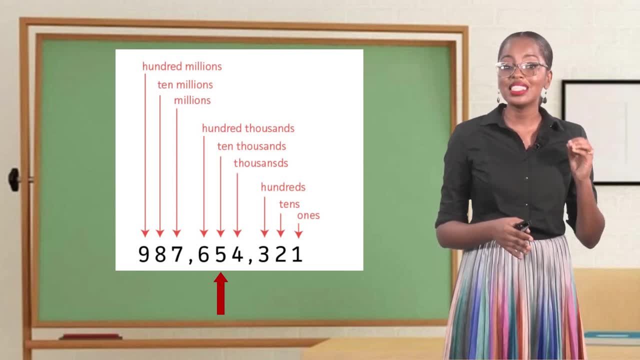 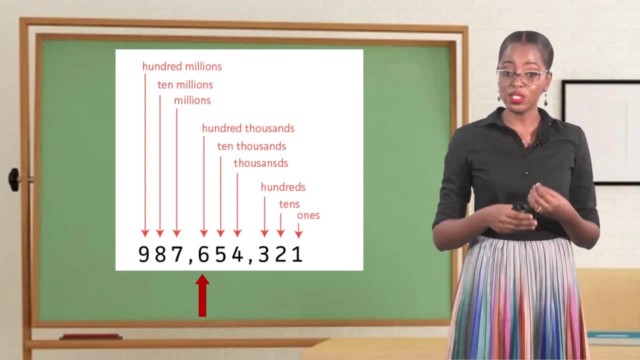 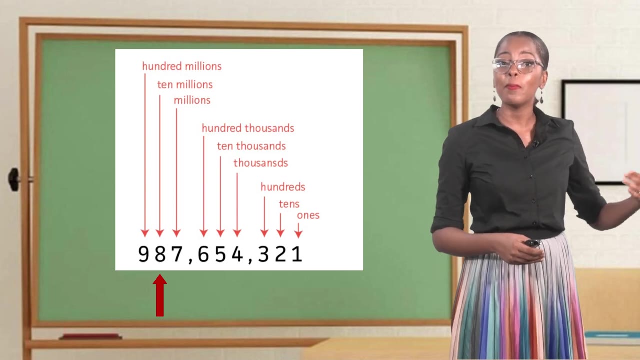 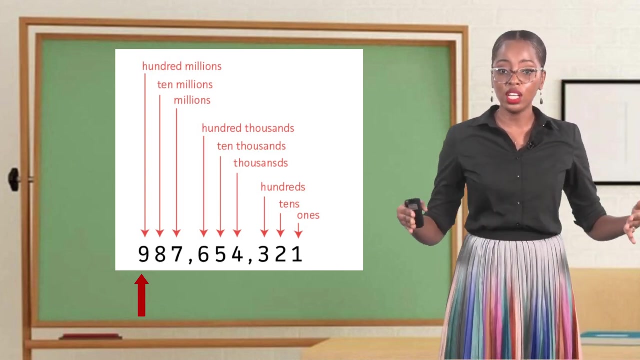 would be ten thousands, Ten thousands and then scheduld, just after ten thousands we have hundred thousands and then beyond that is millions, and then after that would be 10 millions, and then after that we have 100 millions. so the place value it goes on. 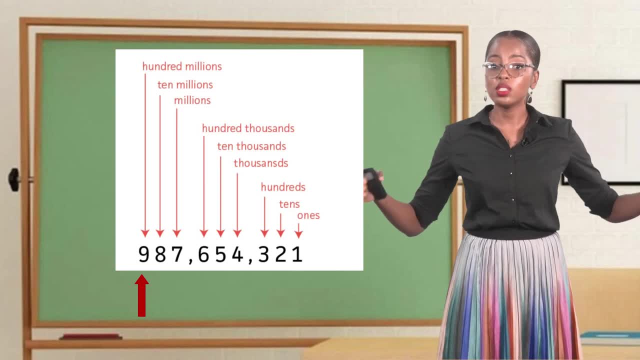 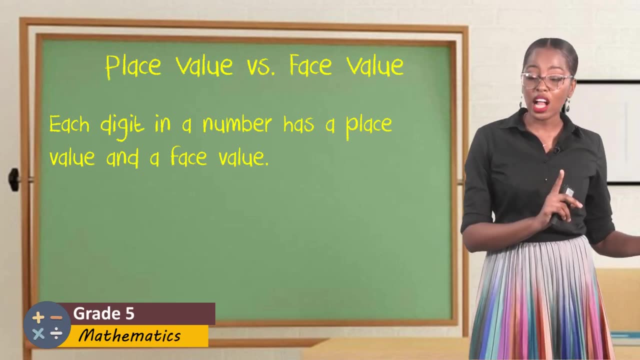 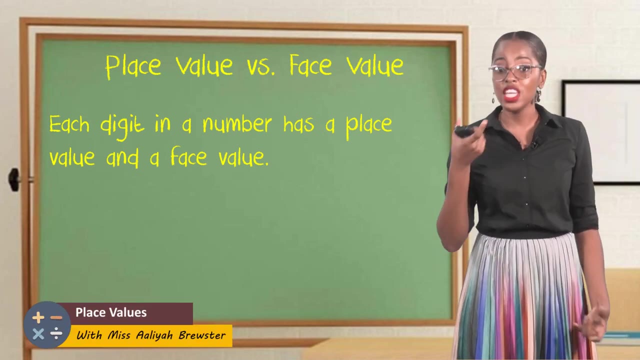 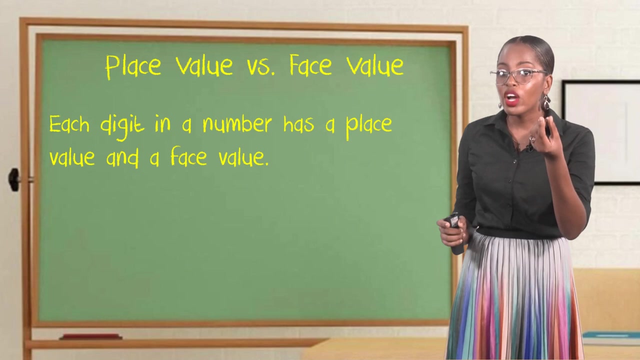 and on, and as the, as the numbers get bigger, so does the place value it holds. now, boys and girls, let's move on to discuss the difference between place value and face value. you see, every number has its place value and its face value. place value would suggest the value that the number 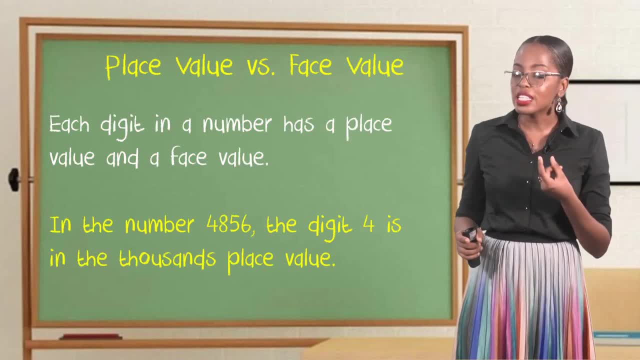 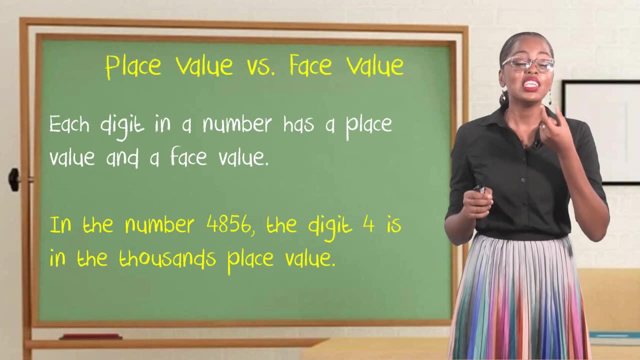 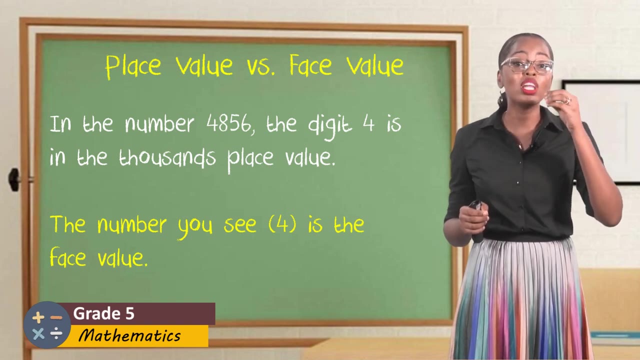 is occupying in a certain place. for example, if we look at the number 4856, 4, there is taking up the place value of thousands. however, if we were asked to identify what, then what is the face value for the number four in that entire number? the face value would be for: 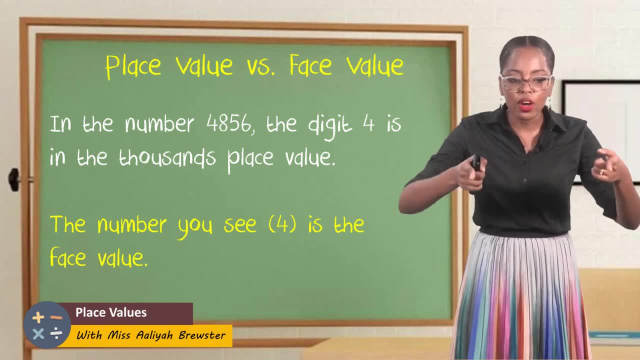 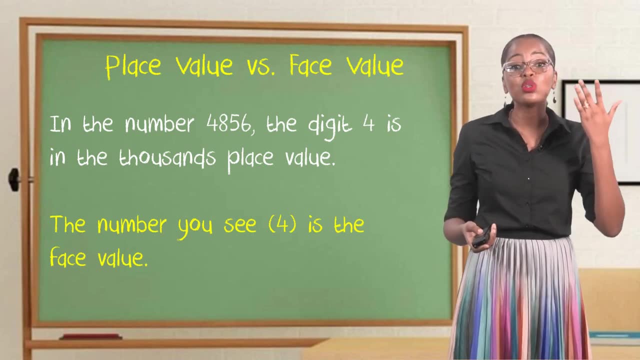 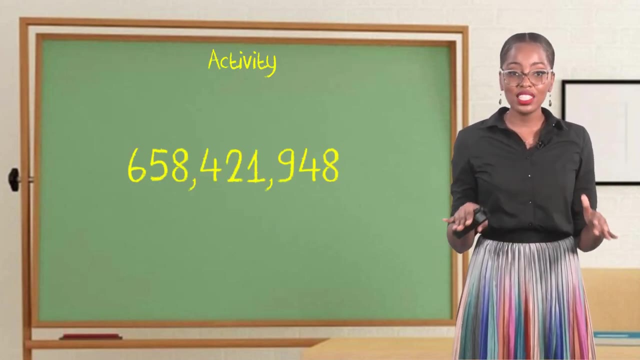 itself, because four is the is the number that is in that place. therefore, it's the face of the thousand value. so the face value is actually the same as the number itself. I have an activity here for you, boys and girls. it's quite simple and I know you'll get it correct. we're going to examine the number 658 million four. 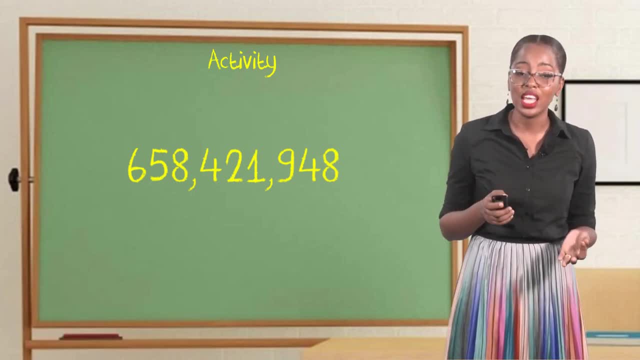 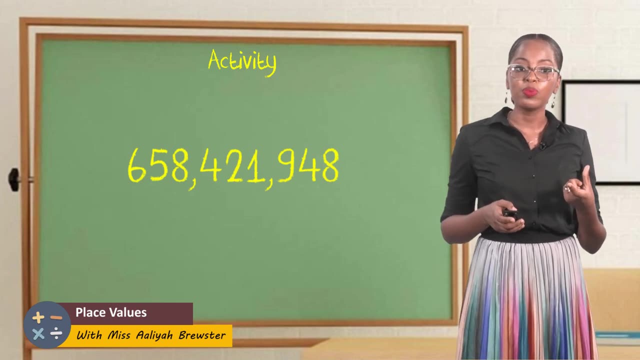 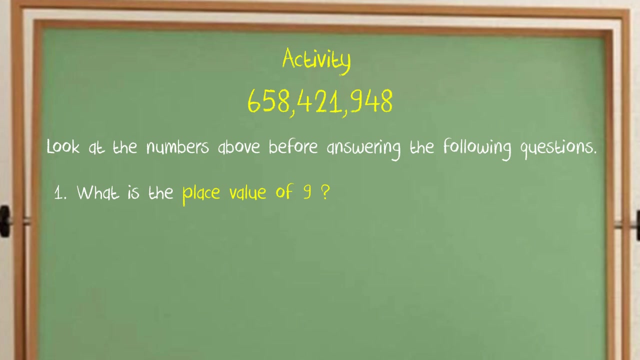 hundred and twenty one thousand nine hundred and forty eight. what we're going to do, we're going to look at that number and then we're gonna answer questions based on that number. the first question is: what is the place value of nine? what is the place value of nine? 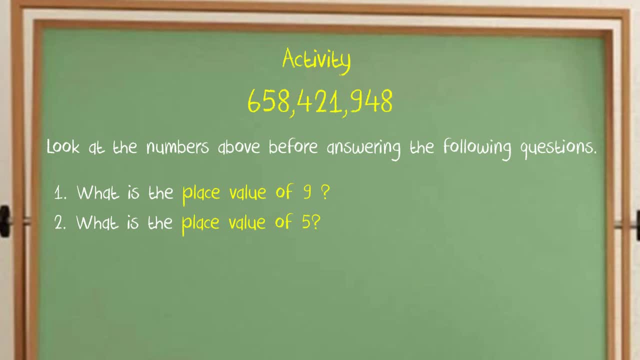 the second one is: what is the place value of 5? what is the place value of 5? and the third one is: which number is in the place value of millions? which number is in the place value of millions? and the fourth question is: which number is? 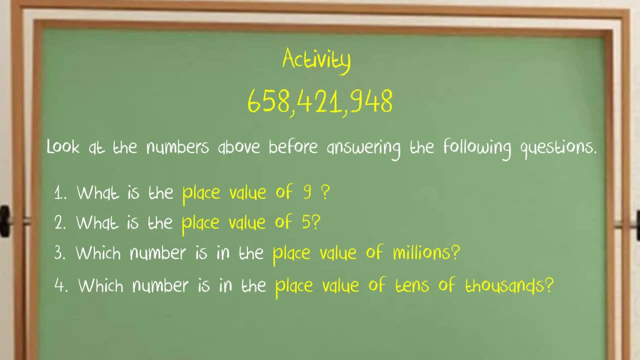 in the place value of tens of thousands. which number is in the place value of tens of thousands? and then the final question is: what is the face value of 6 in the number? what is the place value of 6 in that number? so, so, so, so. 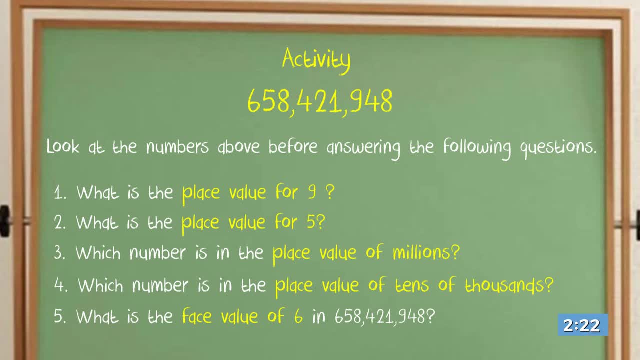 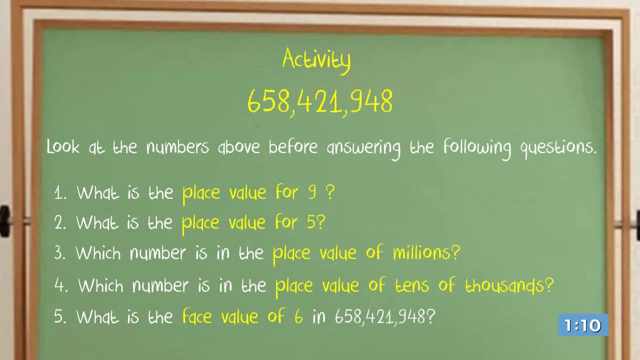 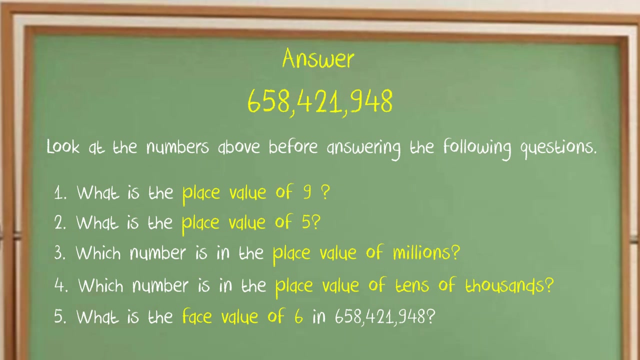 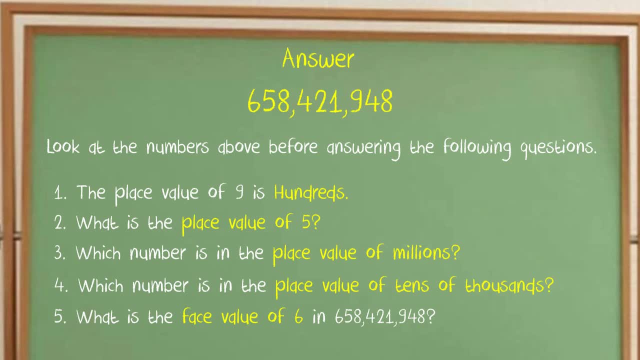 the hundreds place value. For number two, we were asked to calculate a place value for five. Of course, the place value for five is tens of millions. That's right, tens of millions. For number three, we were asked which number is in the place value of millions, and that would be the number. 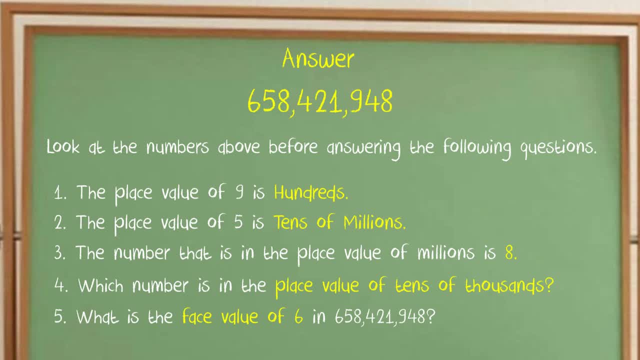 eight. For number four, we were asked which number is in the place value of tens of thousands, and that would be the number two. Well, for the final question, what is the face value of six in that number? and the answer, of course there would be six. Thank you, boys and girls, for tuning in, but 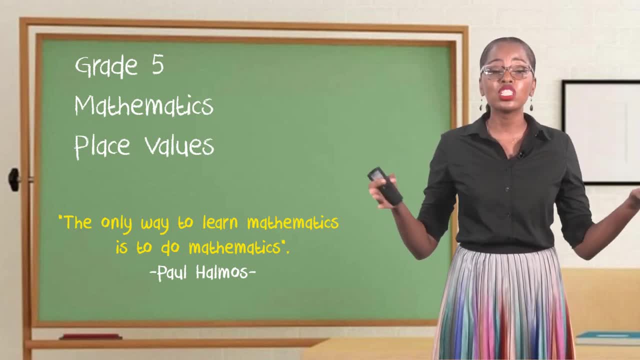 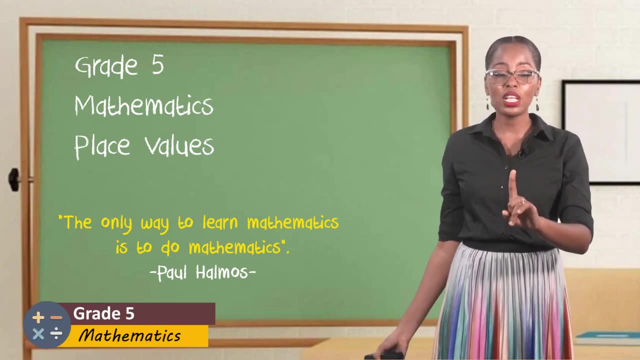 that has brought us to the end of another lesson. I trust that you would have enjoyed it and remember the words of Paul Halmos: the only way to learn mathematics is to do mathematics. So this means that even though our study time might be over, that does not mean that you have to stop practicing. 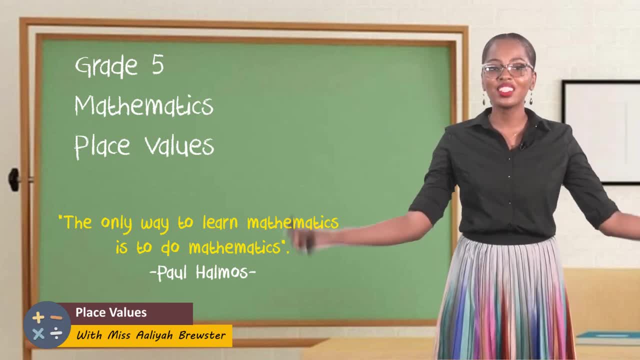 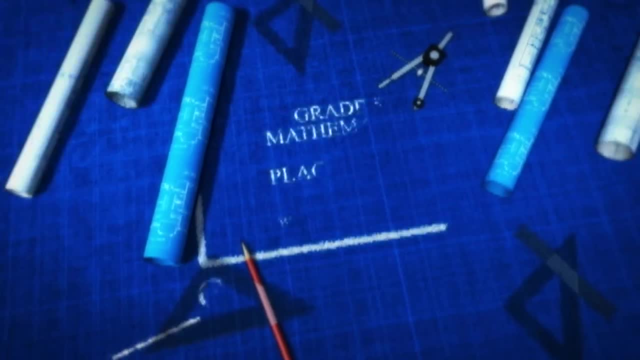 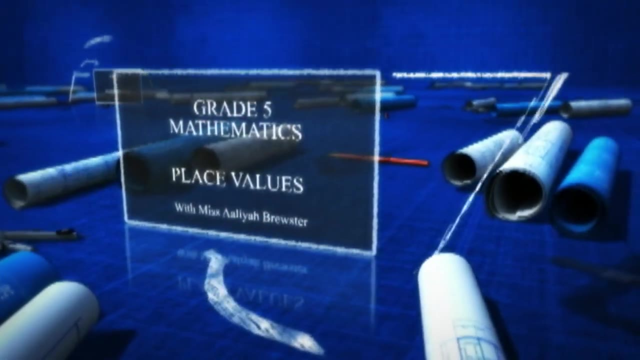 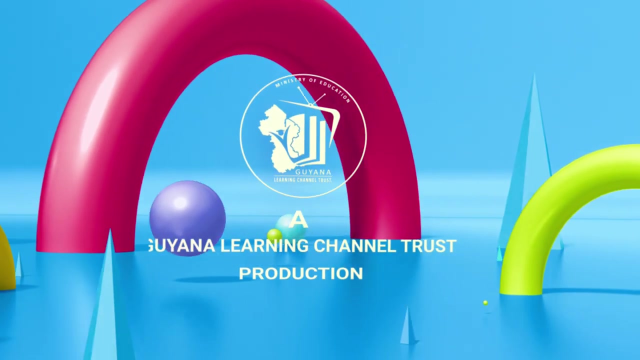 Thank you once again, boys and girls, and goodbye you.